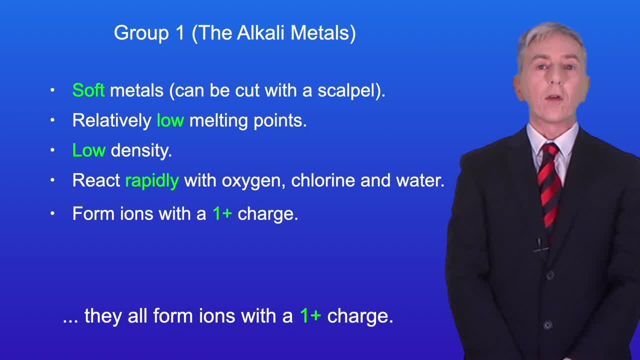 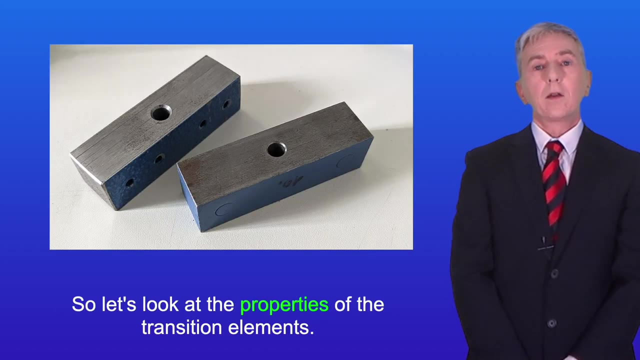 And finally, when the alkali metals react, they all form ions with a one positive charge. So in this video we're going to look at the transition elements and compare them with the alkali metals on group one. I'm showing you here an example of a transition element. This is iron. 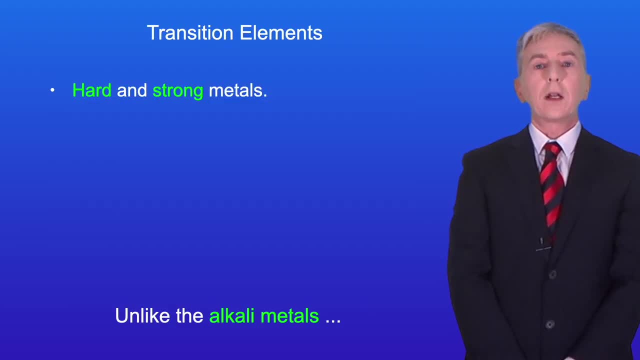 So let's look at the properties of the transition elements. Unlike the alkali metals, the transition elements are hard and strong metals. Transition elements all have high melting points, so they require a high temperature to melt. The exception to this is mercury, which is a liquid at room temperature. 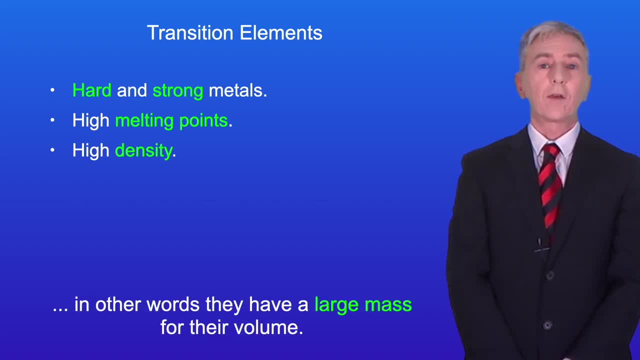 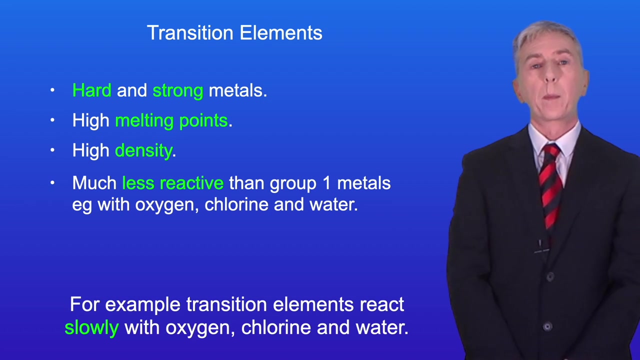 Transition elements also have a high density, In other words, they have a large mass for their volume. Now, if we look at the reactivity of the transition elements, we can see that they're much less reactive than group one metals, For example. transition elements react slowly with oxygen, chlorine and water. 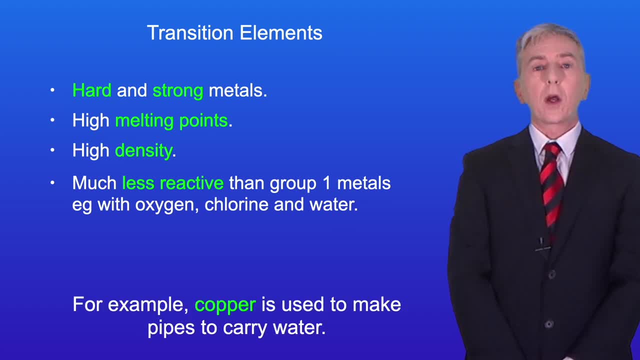 This rate of reactivity makes transition elements very useful. For example, copper is used to make pipes to carry water. Now, just like the alkali metals, when transition elements react, they lose electrons to form ions with a positive charge. However, unlike the alkali metals, transition elements can form ions with different charges. 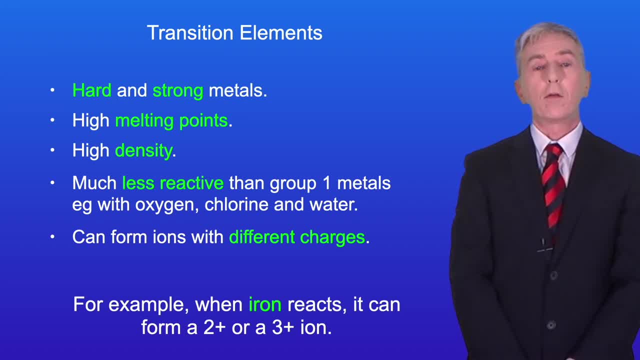 For example, when iron reacts, it can form a two positive or a three positive ion, And when nickel reacts, it can form a two positive ion positive or a 4 positive ion. Another property of transition elements is that they form coloured compounds, and I'm 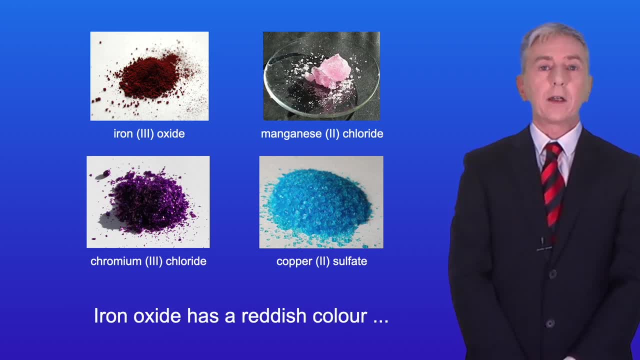 showing you some examples here: Iron oxide has a reddish colour, whereas manganese chloride is pink, Chromium chloride is purple and copper sulphate is blue. Now, the final property of transition elements is that they can be useful as catalysts. Catalysts are often used in chemistry to increase the rate of chemical reactions and in later 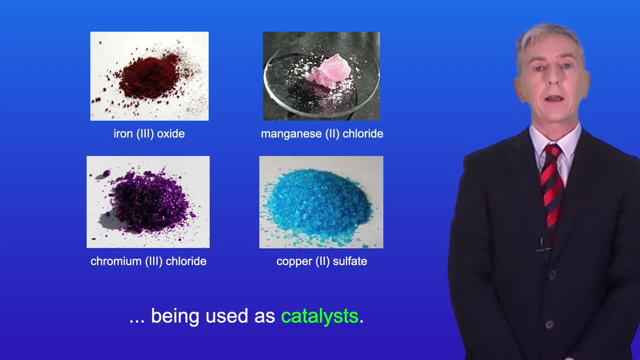 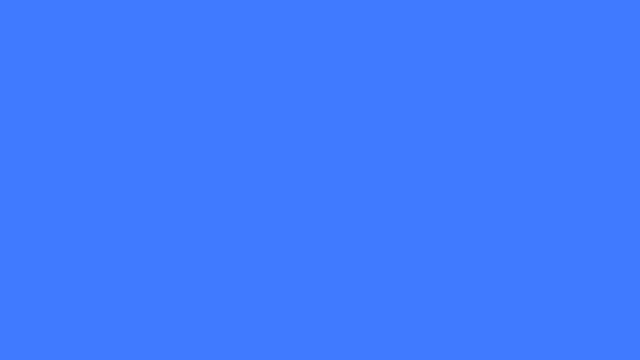 videos we'll see examples of the transition elements being used as catalysts. You'll find plenty of questions on this topic in my Vision workbook, which you can get by clicking on the link above.